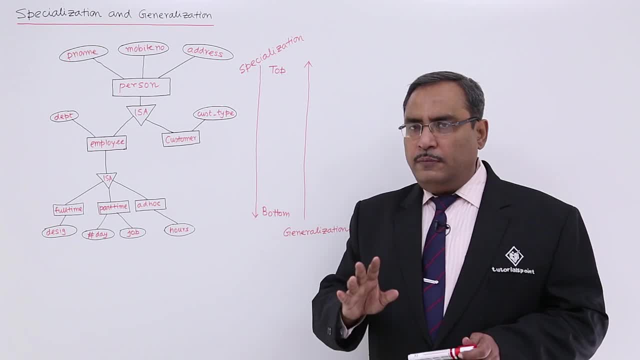 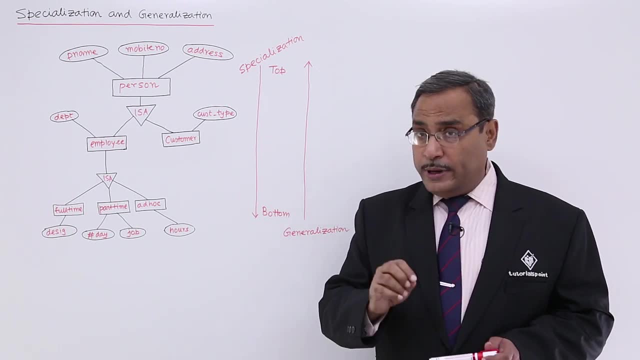 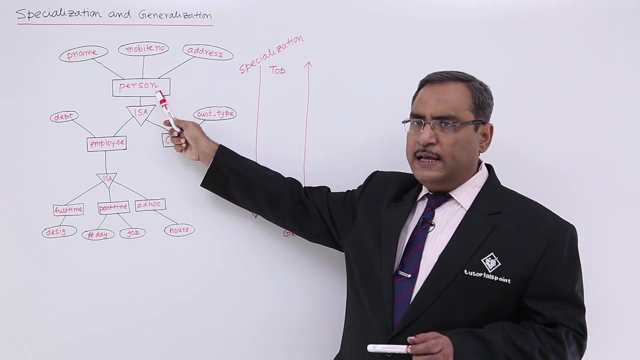 ok, now thing is that i shall not form, or i should not form, tables or schemas against all entities. what will be doing, you see, whenever this person has got is a so against person, i shall not draw any kind of schema or table, but this leaf in this particular tree, this 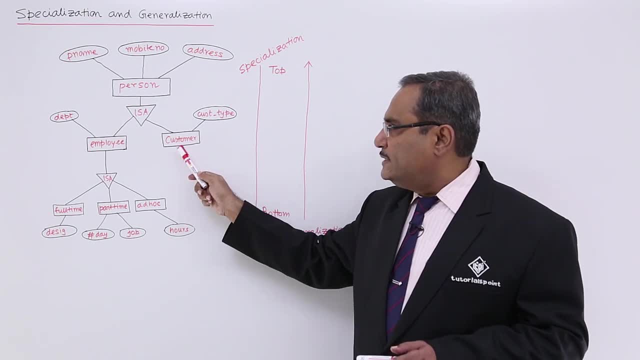 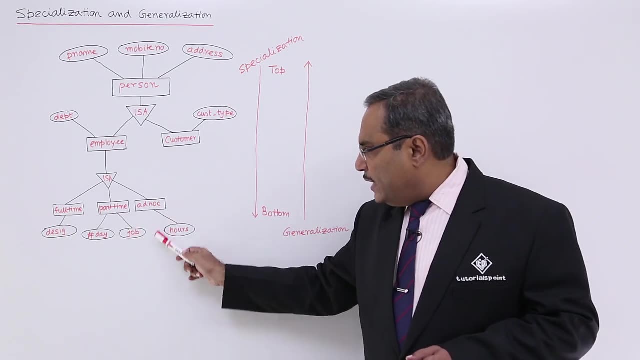 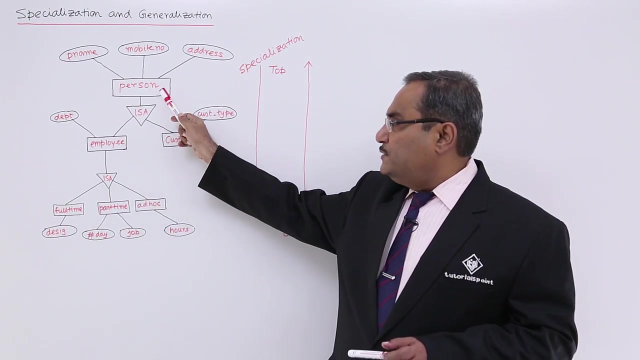 is the leaf entity, because from here that is no is a, this, this one, this one and this one, all these three are the leaf entities. from where that is no is a this employee is having is a, i shall not form any table against this employee. this person is having is a. so 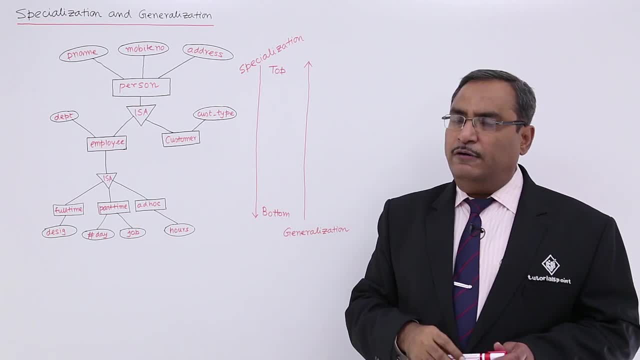 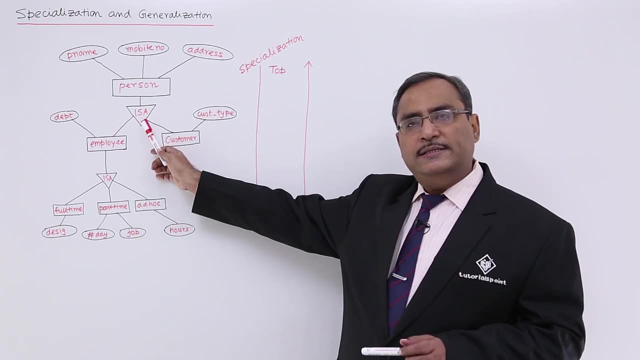 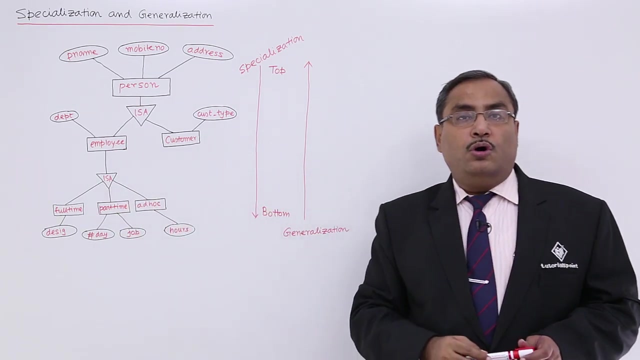 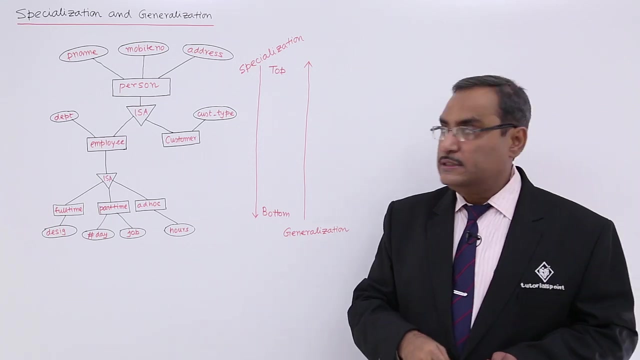 this person, against this person, i shall not form any kind of entity, any kind of schema or any kind of table for that. so this is my table. specialization has been done and for it specialization has been done. so how to get the attributes of those entities for which i am going to form the tables or schemas? so for customer. 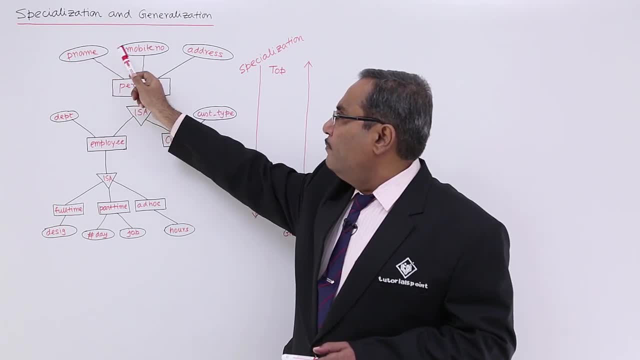 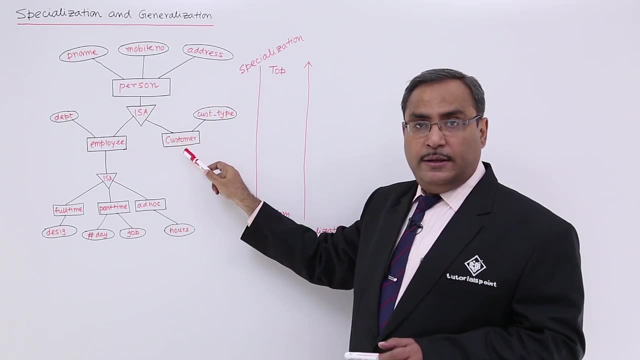 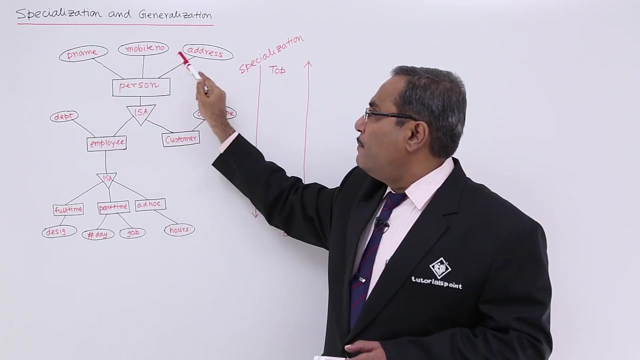 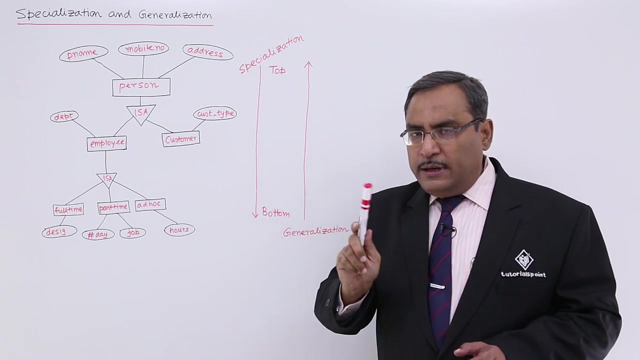 the attributes will be person name, mobile number, address and customer type. so you see, these particular attributes are getting inherited and this customer is getting those attributes through attribute inheritance. so this is my person name, mobile number, address and customer type will be coming for customer, for employees, i'm not going to form any schema or 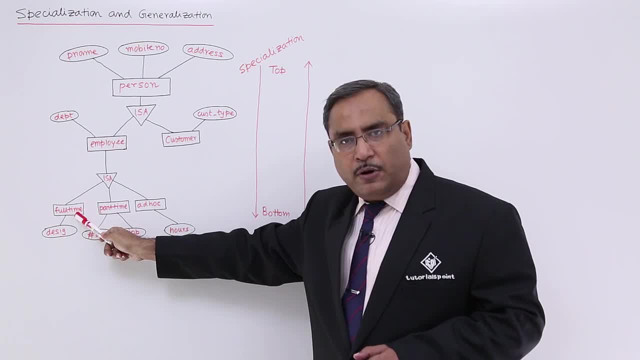 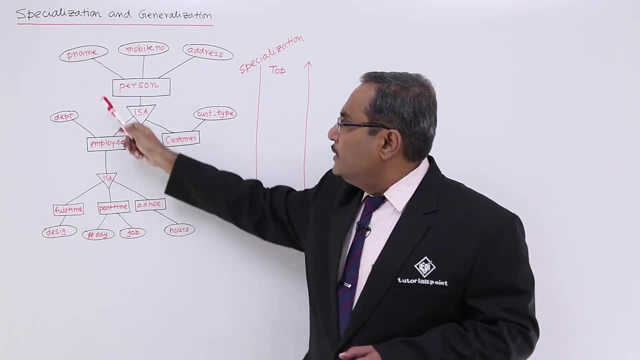 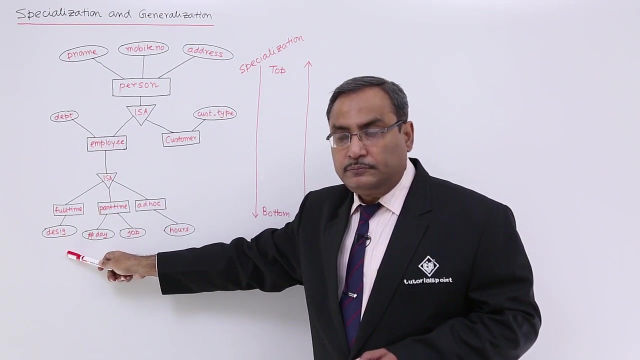 table. so for employees i'm not forming, but for full time i'm forming because there is no specialization here, there is no easy here. so full time we'll have just see here there is a person, name, mobile number, address, department and this designation and this part-time will have part-time. 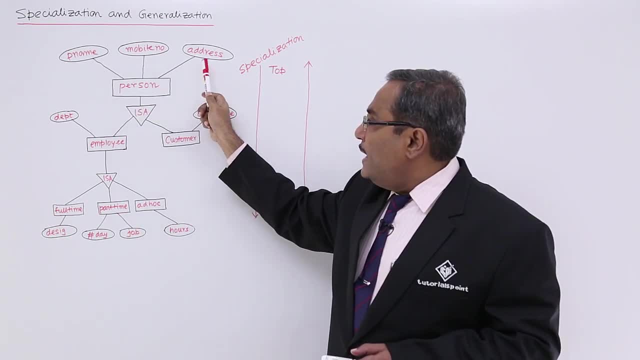 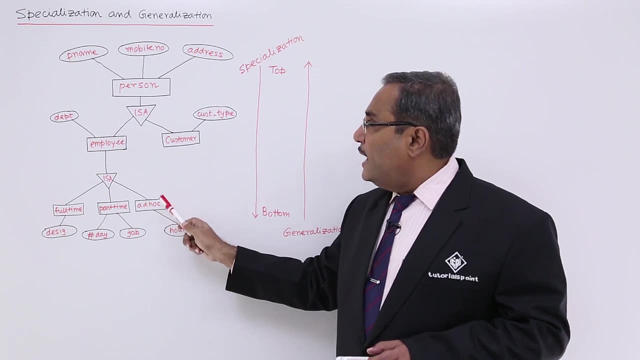 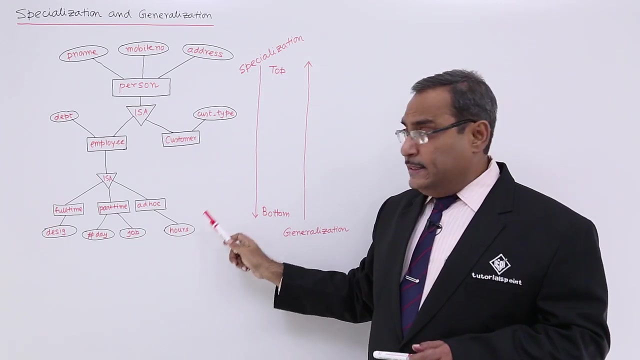 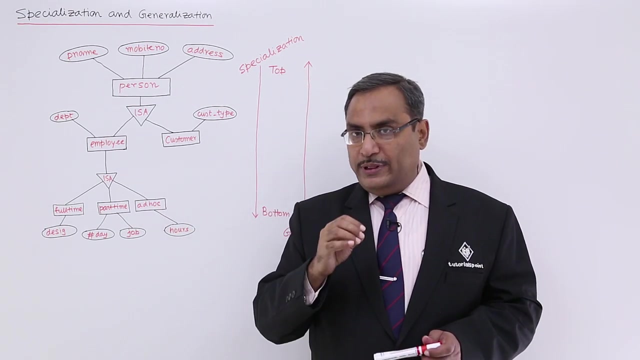 employees will have person name, mobile number, address, department, number of days worked and the job title. this ad hoc will have person name, mobile number, address, department and then hours worked. so in this way, one, two, three, four, so four schemas and against four tables will be formed with these mentioned attributes. so if you move from top to 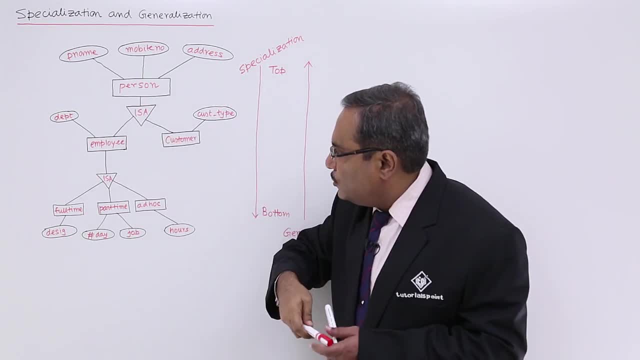 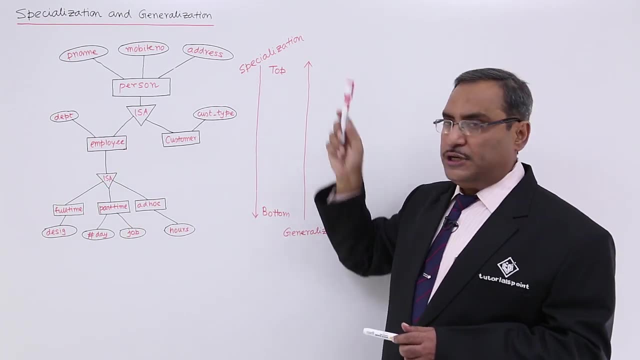 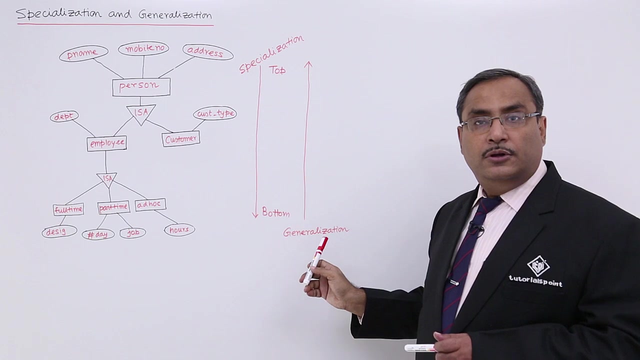 bottom. in this way, you are going to get easy in this way. so i'm getting person, is getting two types of, that is, employee and customer. so it is known as specialization. and if you move in the reverse order, that means from the bottom to the top, then it is becoming generalization. so here, 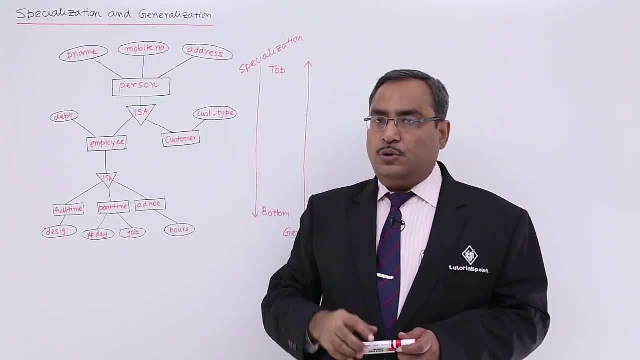 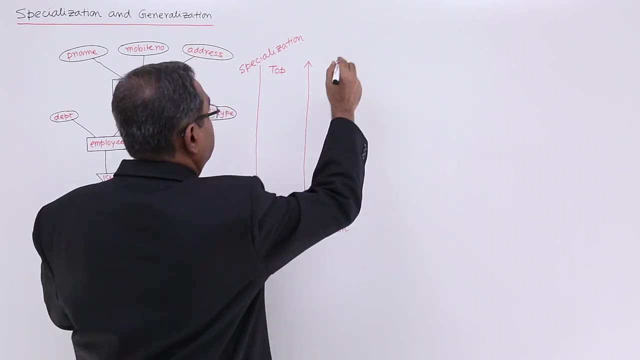 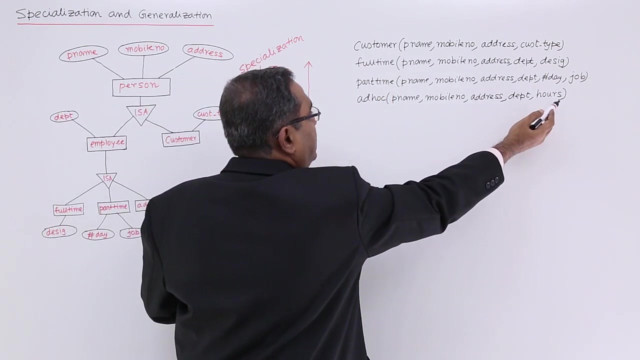 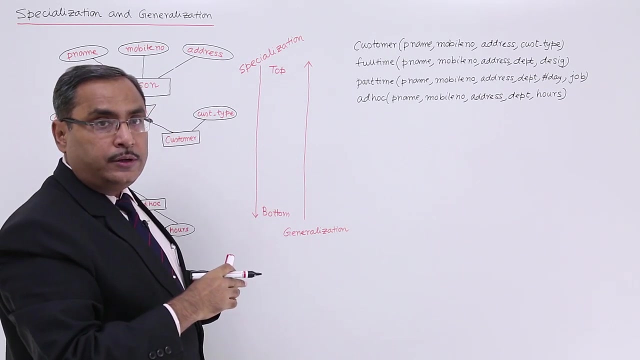 we have explained this one with the proper example, so let me write the respective schemas for you and in this way see. so these are the four schemas and with the respective attributes, whatever we have discussed earlier. accordingly, we have written this one. so: customer- full-time, part-time and. 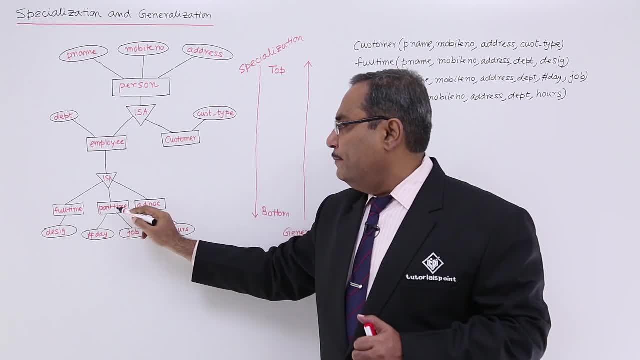 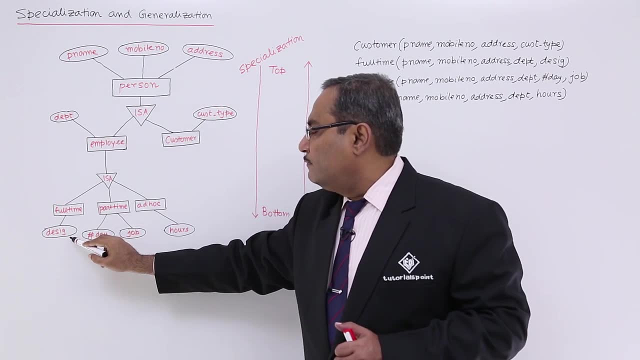 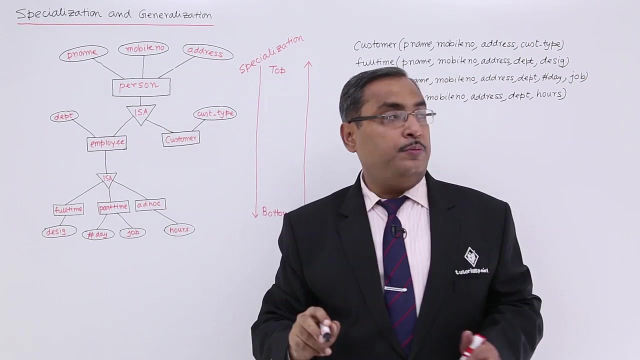 ad hoc. you can see here customer, full-time, part-time and ad hoc customer with the four attributes. this full-time will be four plus one, five attributes, part-time will be four plus two, six attributes. and ad hoc will be this: four plus one, five attributes. and i have written them. 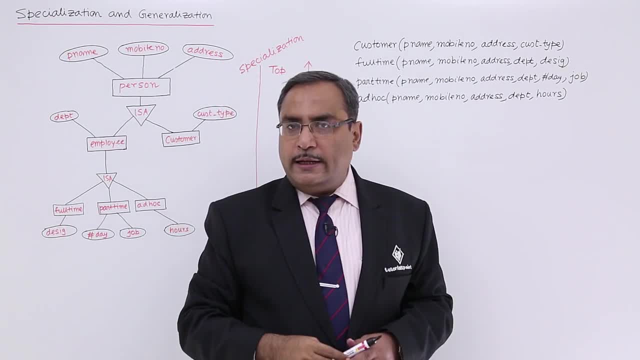 in the respective order also. so i think you are getting this particular logic how the tables can be formed from such year diagrams. thanks for watching this video. 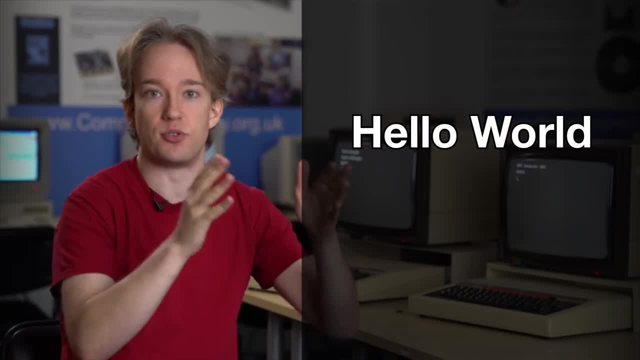 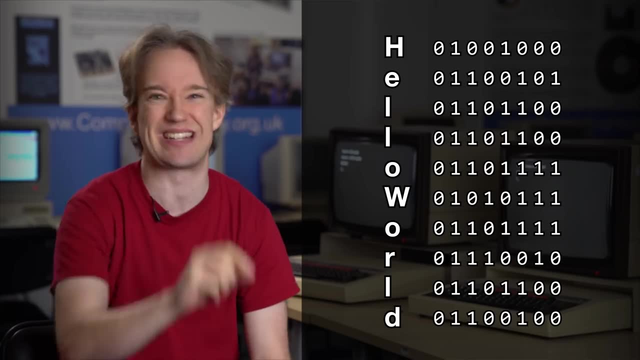 When you put English text into a computer, it is saving every individual character as eight bits of data, Eight ones and zeros. I mean, they're not actually ones and zeros, they are particular positions of atoms on a disc or a few electrons going over a wire. but as far as we're concerned, in the computer, 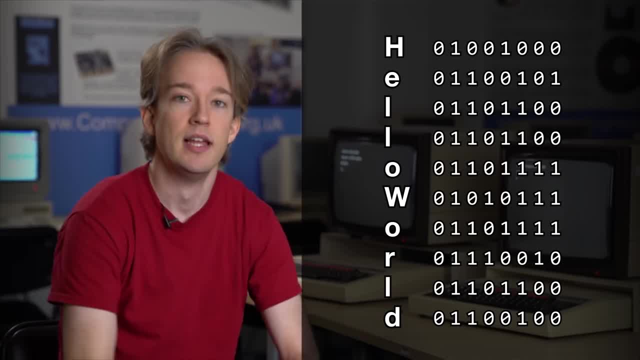 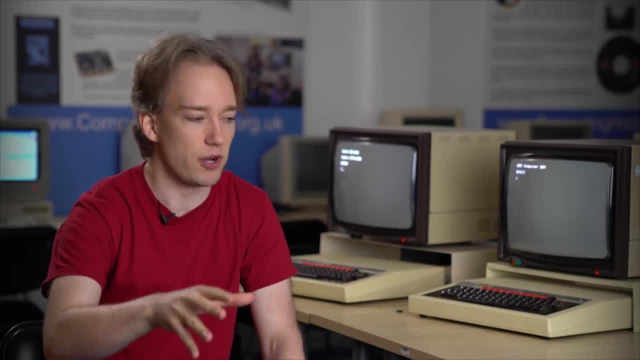 science world. they are ones and zeros Bits, And, yes, a modern phone or computer might store a few quadrillion of them. but every time you've had to wait a long time for a download or your phone has complained that its storage is full, you are running up against the same question that computer scientists. 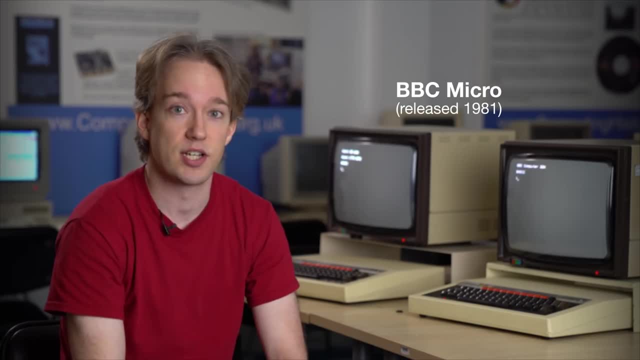 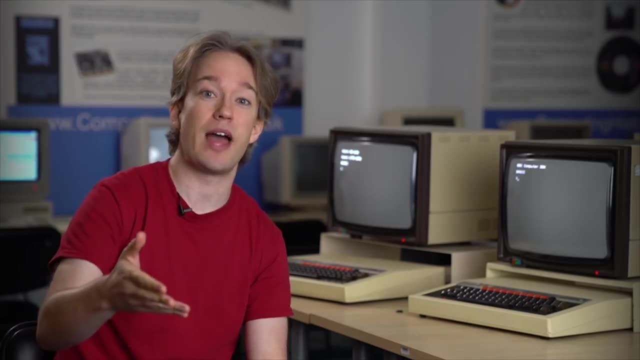 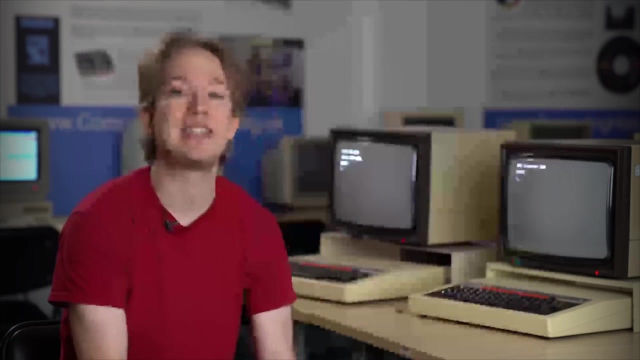 have been working on since before. These things here were state-of-the-art. Can we please not use so many bits? So let's run through how computers compress text. Images and video are different. that's lossy compression, where it doesn't matter if you lose a little bit of detail, But text.